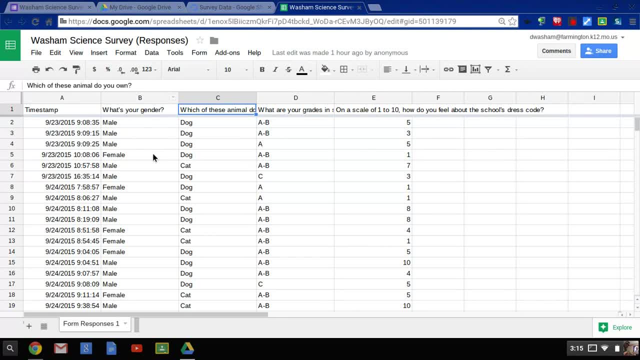 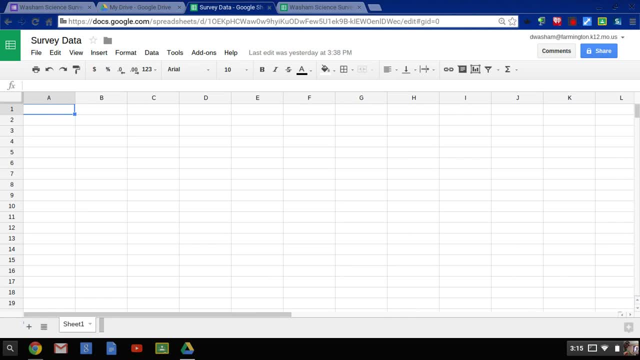 to go to my independent variable, which in this case was gender, And for gender there's only two options: male or female. And so I'll go to my sheet and I'm going to title my independent variable gender. And then I had two options: male and female. Now again, whatever your independent variable, 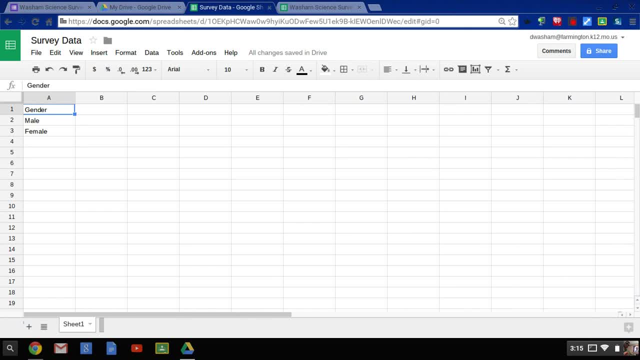 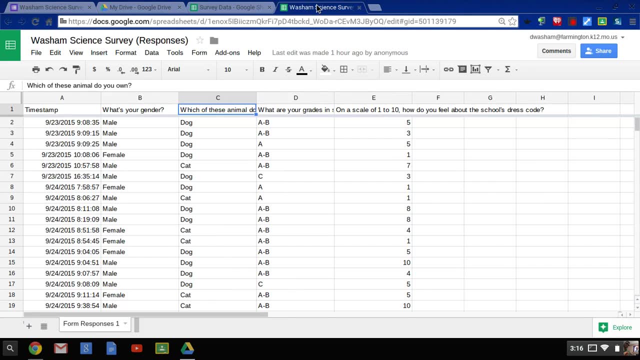 was, it could be something completely different than gender. You would give the title of it there and the options going down in the first column. Now, next to it, in the next column, over, I'm going to look at my independent variable And I'm going to go ahead and click on the data And I'm going 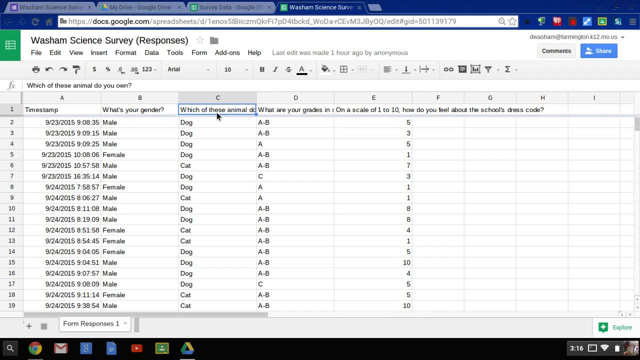 to go ahead and click on my independent variable And I'm going to go ahead and click on the data And I'm going to go ahead and click on the data And I'm going to go ahead and click on the data And the first deep in a variable which was: which of these animals do you own? Again, I do not know. 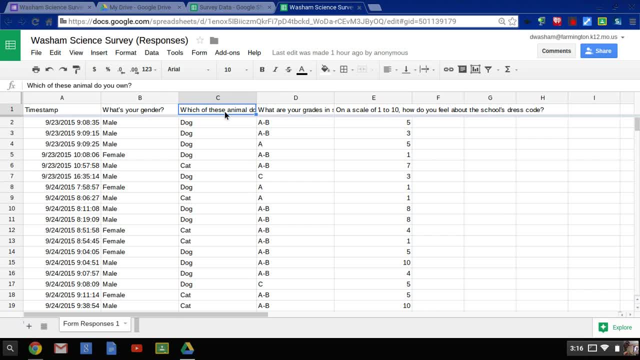 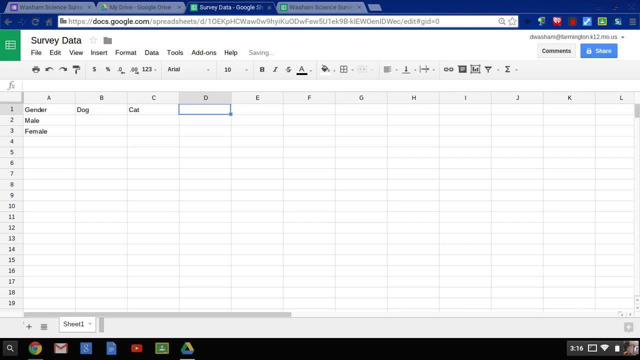 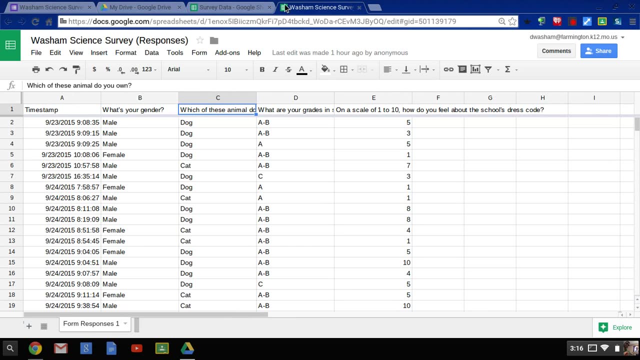 what your group asked, But in this situation they were asking about animals, And so I'm going to put the possible responses- dog, cat, horse- here and I'll continue. if there's more responses in that, I would fill those in And then I'll just have to go back to the data And I've just got to count up. 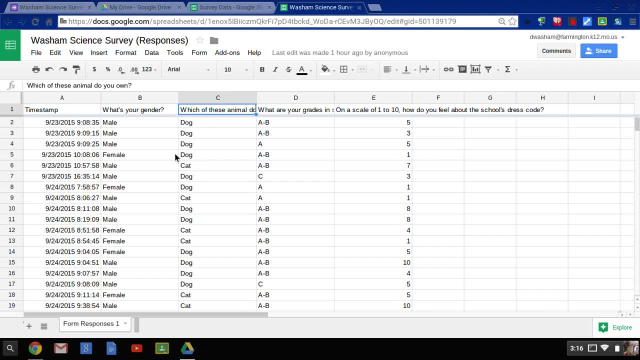 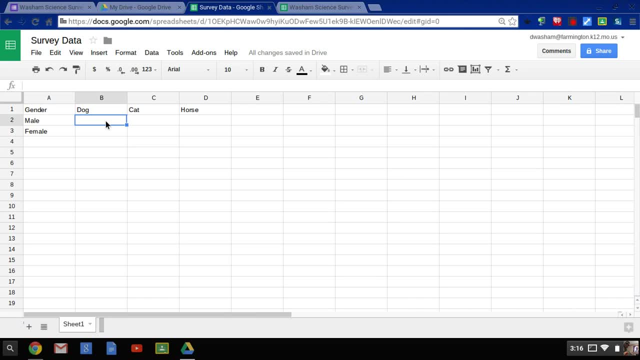 real quickly. You know how many males said dog, how many females said dog, how many males said cat, female said cat and so on. And as I'm getting my data gathered, I just type in the answers here. So let's just say that there were 12 males that said dog and 13 females And under cat there. 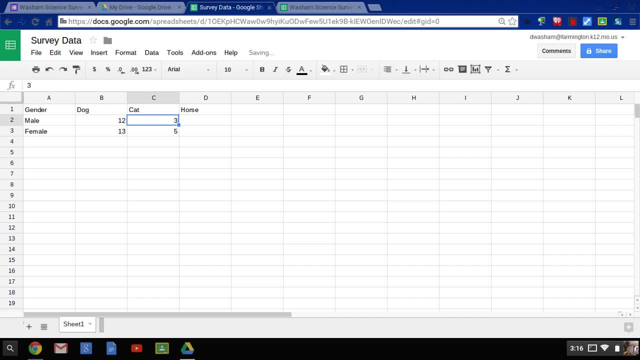 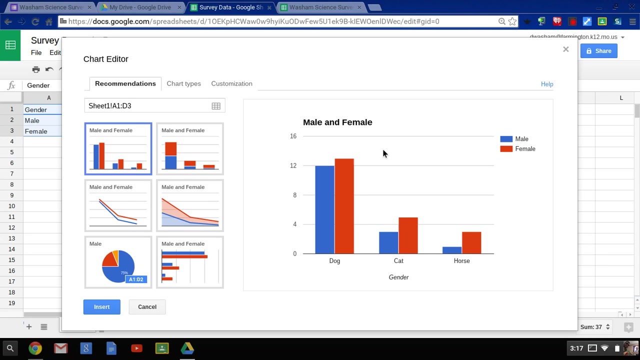 were three and five And under horse it was one and three. Alright, so there were the answers that we received, And to turn that into a graph, I just select everything, I go to my insert chart And it's probably going to produce a bar graph for you, which in this case, is fine. I know, we are only 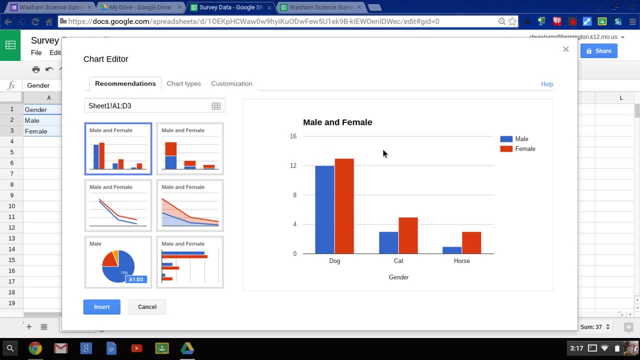 doing line graphs in class, But this sort of day that we're getting back from our classmates is really hard to turn into a line graph. So this shows up really nice and neat. It shows males, females, it shows the number that responded for dog, cat, horse. It's a very easy graph. 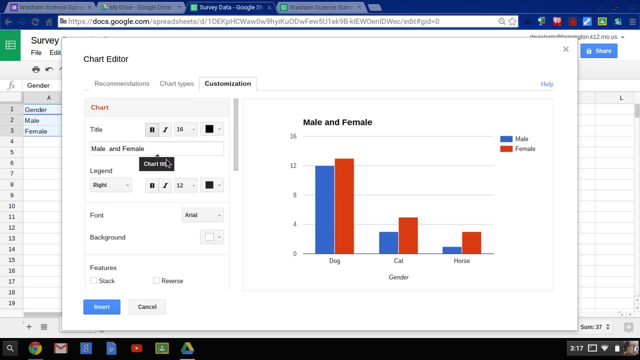 I'll just need to go to customization And make sure I have an appropriate title. probably starts with something like the effect of you do want your legend, And then you can go to your left vertical And you can go over to your left vertical and you can. 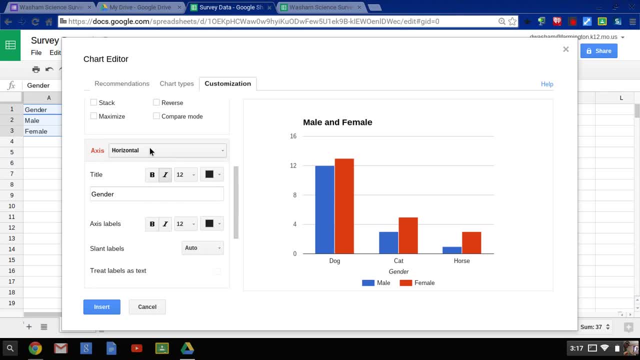 go to your left horizontal axis and you can go down to the axis and change the label of the horizontal axis And right now it's set to gender. obviously you'd want to fix that to be the correct title, and then you can switch it over to your left vertical And you can fix the title of your left. 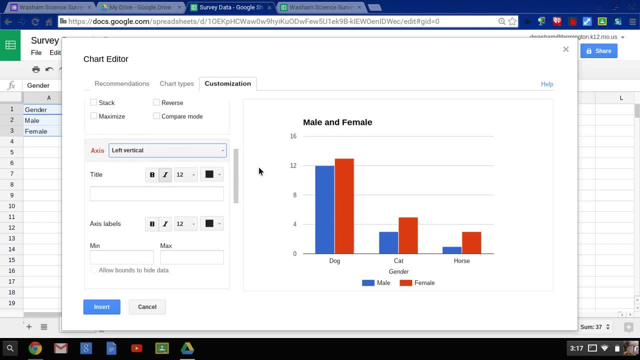 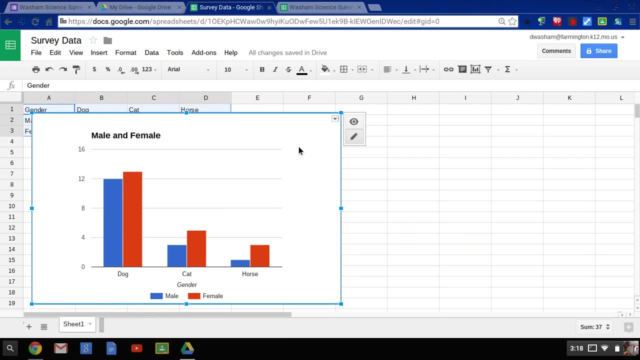 vertical axis. Once your graph is correct, with a title and label for the axis, you can go ahead and insert it into your graph, into your data table or into your sheet. excuse me, and you can just go ahead and, on this button, choose the down and say move to own sheet and it's just going to stick it in there. nice, and 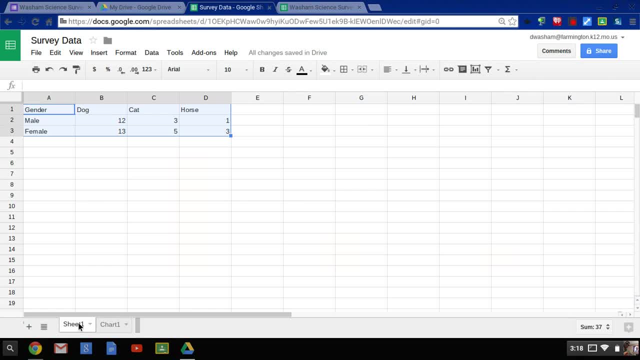 big for you in its own sheet. You click back on sheet one and your data is still there. Now you're going to do the same thing for the other question. So remember you have the same independent variable every time- gender- and my options were male and female, and but this time I'm going to go to the 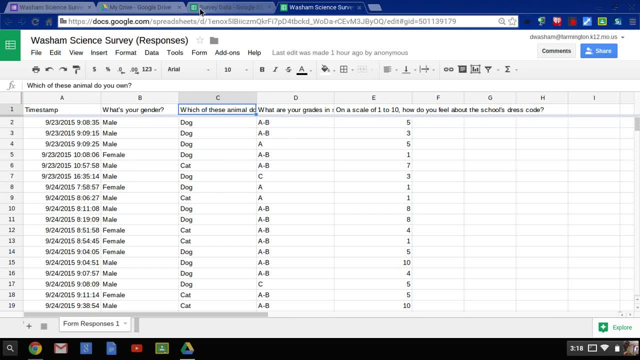 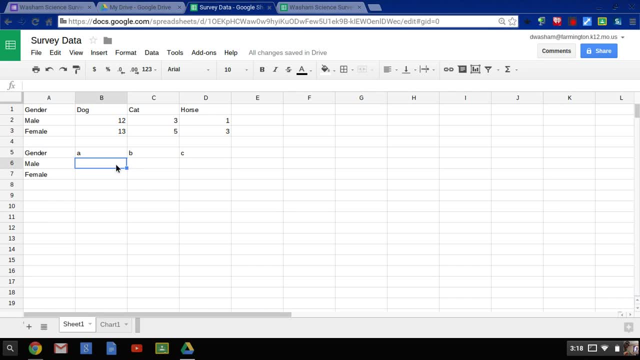 second question, and on the second question is: what were your grades? and so I would again put in my possible responses that students could answer. from so on, I'll go and do the counting and I'll put in the numbers here, and as I put in those numbers, 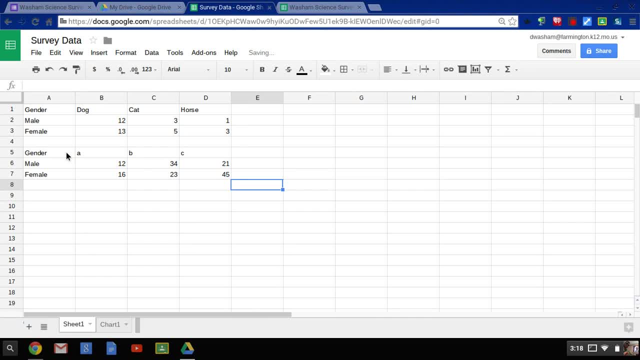 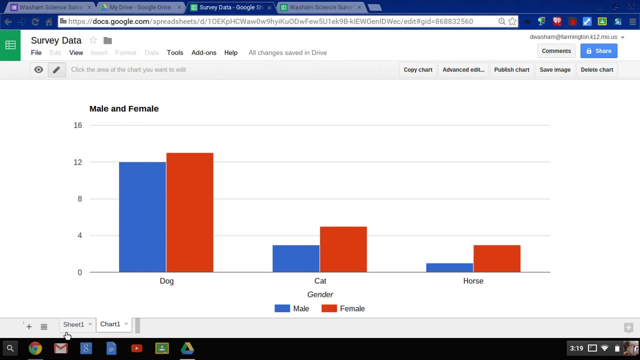 I would go and select everything- same process- make a graph and again it's going to make a graph for me. same process: I insert into the sheet and once it's made and then I move it to its own sheet. Once that is done and done for you, and you have made all three graphs, because you should have. 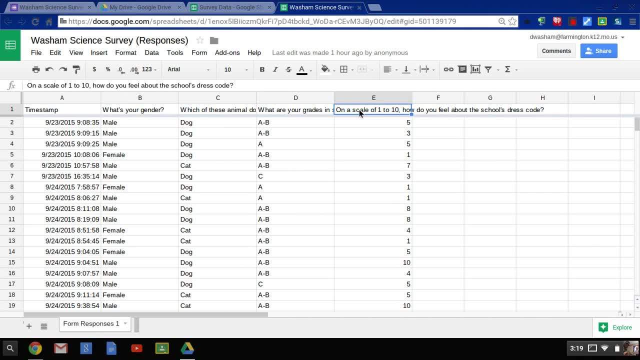 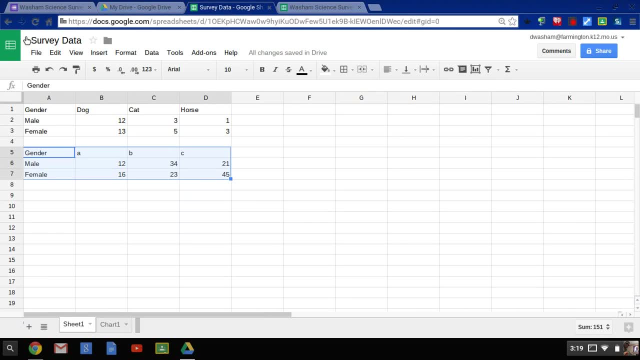 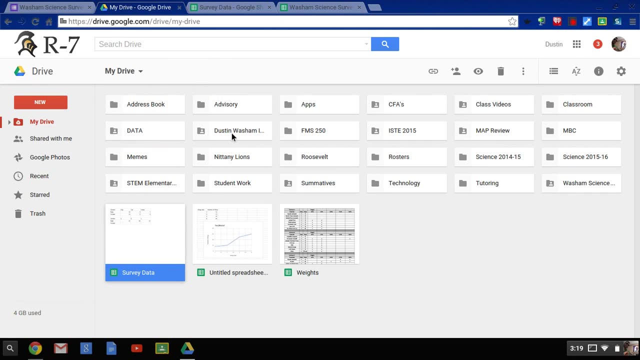 three questions. In this case, what are your grades? and the third one was on the scale of one to ten: How do you feel about the dress code? So, once I've made a graph for all three, I'm going to take that new sheet that I made called survey data and in my Google Drive I'm going to move that sheet. 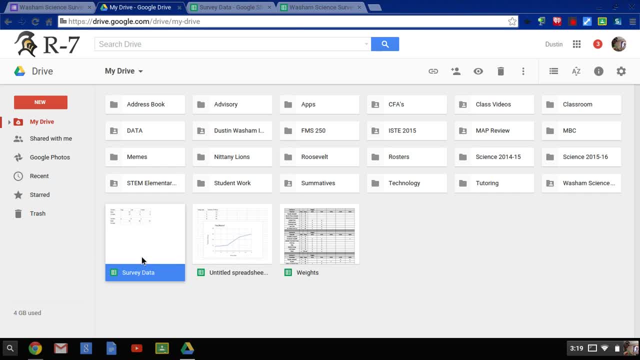 there's survey data. I'm going to take that sheet and I'm going to move it into a folder that's been created for me called science class, and if you need help finding that, let me know. Most of you have already started putting stuff in it, but that is what will turn it into me, So you're going to drag.